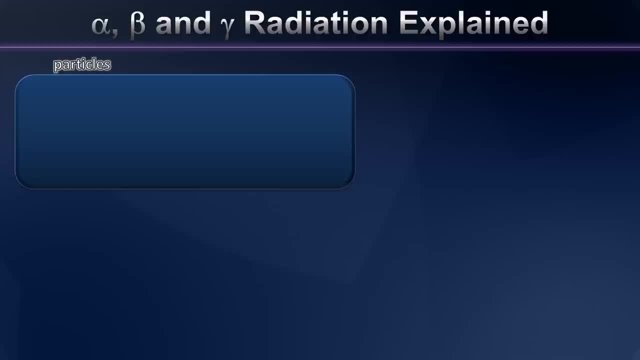 about subatomic particles. Now, we all know the nuclei of atoms contain neutrons and protons, but what you might not have thought about yet is that they can also absorb and release electrons and even photons. And actually there are many more particles that can participate in radiation, but we're going to deal with. 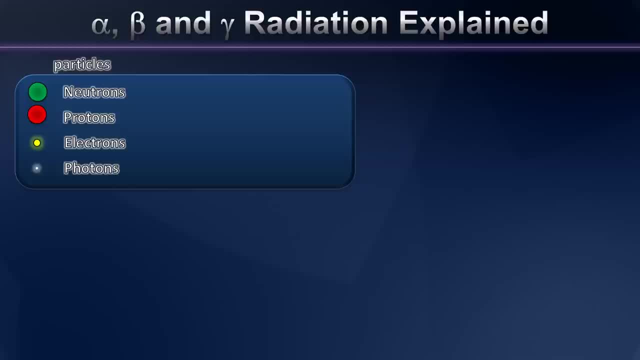 just these four, since we're getting an introductory lecture here. So let's think about all four of these in terms of their charge and their mass. Neutrons, of course, are neutral with a charge of zero. Protons, we know, have a charge of. 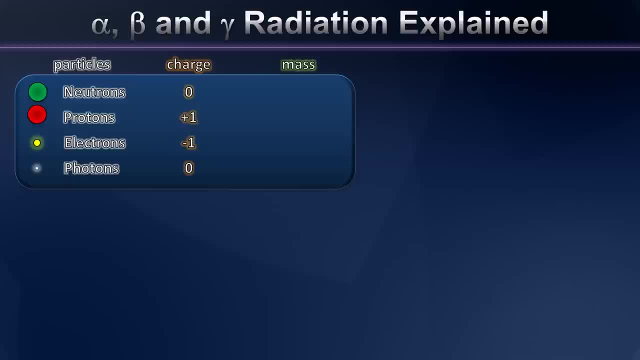 plus one, electrons of minus one, and photons we can think of as having no charge at all. Neutrons have a mass of 1.008701 atomic mass units, and protons are not far behind at 1.007316 atomic mass units. But electrons, well they're so. 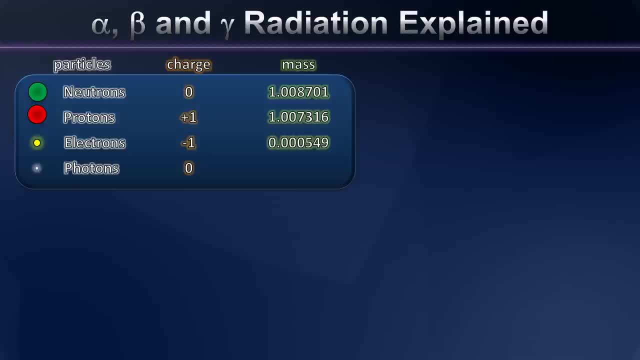 much less massive than protons and neutrons that we typically don't think of them as having mass. When we calculate the mass of an atom, we usually just neglect electrons altogether, And photons. well, photons we think of as being essentially massless. they're so very, very tiny. Now look at this table. 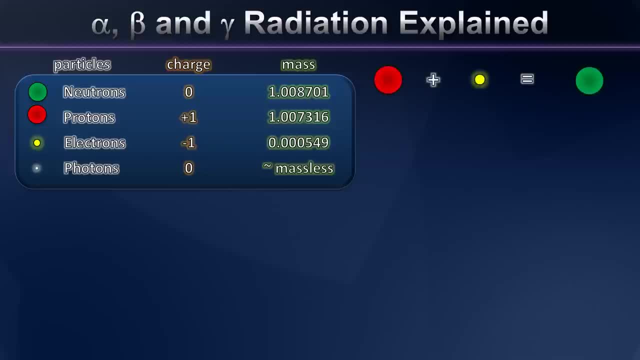 carefully and you'll start to see some relationships here. It kind of seems like a proton plus an electron equals a neutron in a lot of ways, doesn't it? A proton has a plus one charge and an electron a minus one charge, so if you could mix the two together you'd get a charge of zero. just. 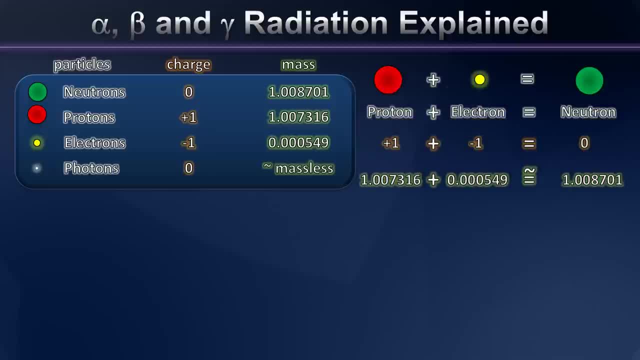 like a neutron has, And although it's not a perfect addition due to something we could actually understand and call the mass defect, a proton plus an electron from a mass perspective does roughly add up to the mass of a neutron, So we're going to use these relationships. 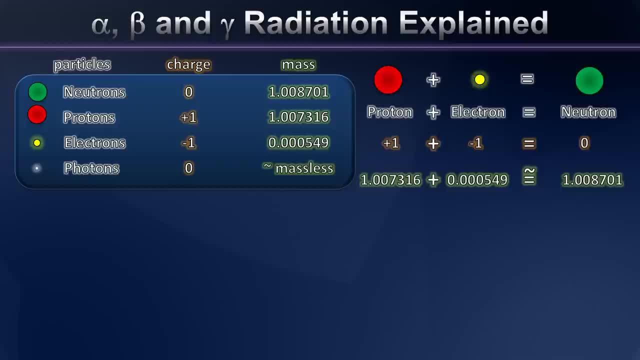 to try to understand nuclear radiation here very, very soon. But enough about subatomic particles. we're here to talk about how atoms behave. So let's think about an atom of uranium. An atom of uranium will have a nucleus with an electron cloud. but again, let's ignore the electron cloud because we're talking. 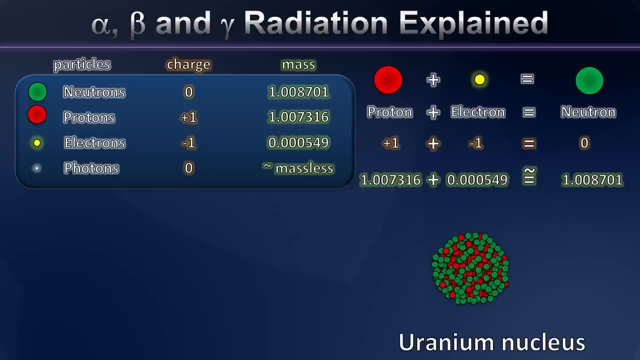 about nuclear chemistry. here We want to talk about the uranium nucleus. A uranium nucleus contains 238 nucleons, or neutrons and protons put together, and 92 protons themselves. This means it has an atomic mass of 238 and an atomic number. 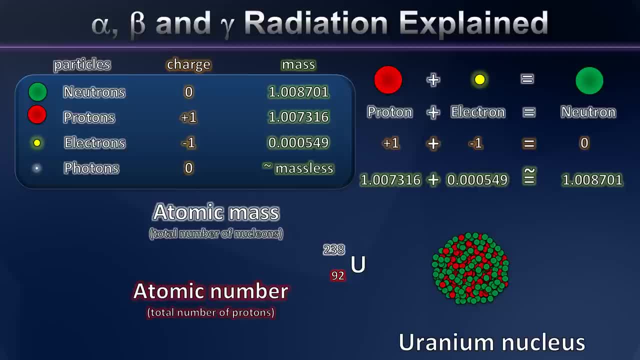 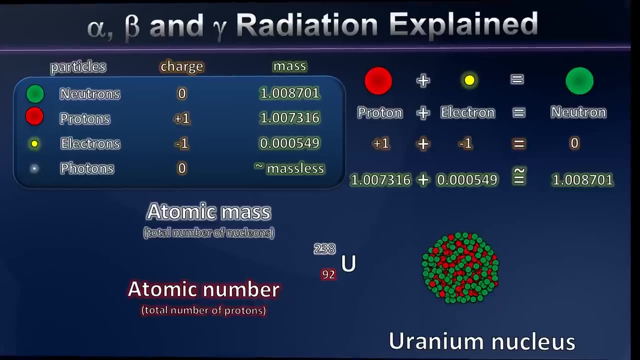 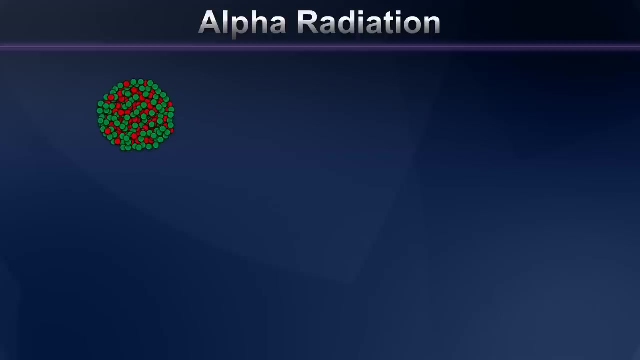 of 92.. It's this uranium nucleus that's going to start our discussion about the concept of nuclear radiation and help us to distinguish between and among alpha, beta and gamma radiation. Let's start working on that right now. First, we're going to talk about alpha radiation, So let's think about 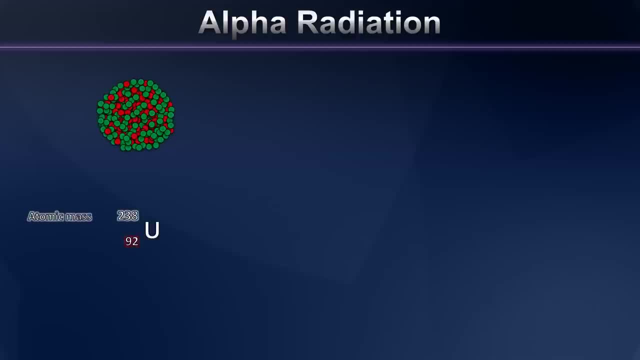 that uranium-238. once more, Remember the atomic mass. 238 tells us the total number of protons and neutrons and its atomic number 92 tells us it's proton number. I'm going to make a duplicate of this nucleus and now it's going to undergo radioactive decay. 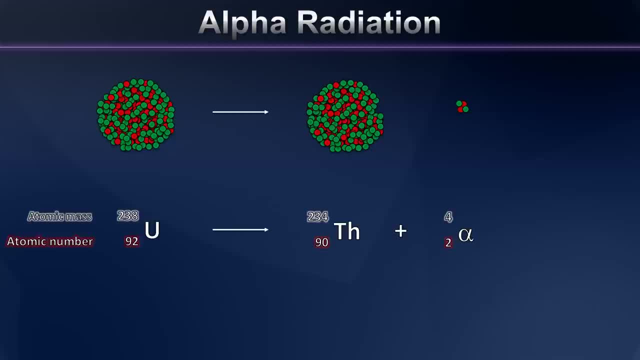 This is an alpha decay. Notice what's come out of my nucleus. I've lost two protons and two neutrons. That means I've essentially lost a helium nucleus. Now look closely at the atomic numbers and atomic masses of all of the parties that are 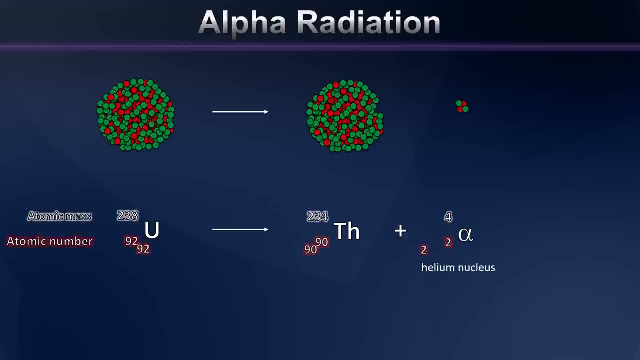 involved here. Notice that the atomic number of uranium-92 is equal to the sum of the two products, thorium and an alpha particle. Notice the atomic masses as well. add up: Charge is balanced and mass is balanced as well. In this case, I've lost a helium nucleus. 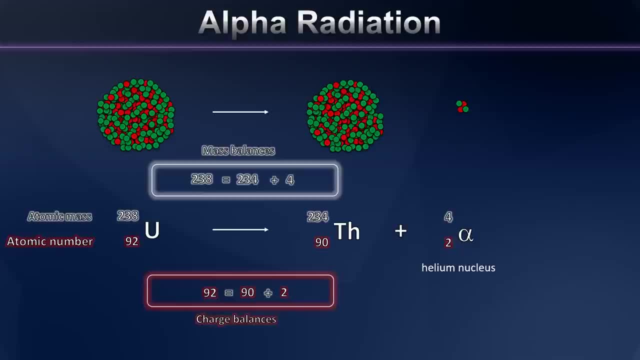 that's four total nucleons and two protons, meaning I have a very massive positively charged particle being irradiated from that nucleus and it's giving me a new atom, a thorium-234, to work with for the next phase step in my radioactive decay. 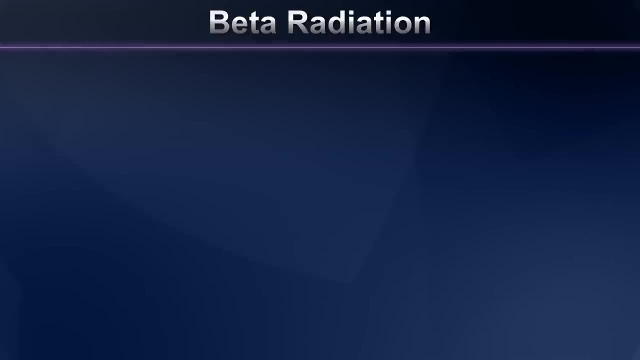 The next step in our process is beta radiation. Now let's think about thorium 234 once more. Its ratio of protons and neutrons has changed as a result of the emission of an alpha particle, and thorium will seek out to fix that In. 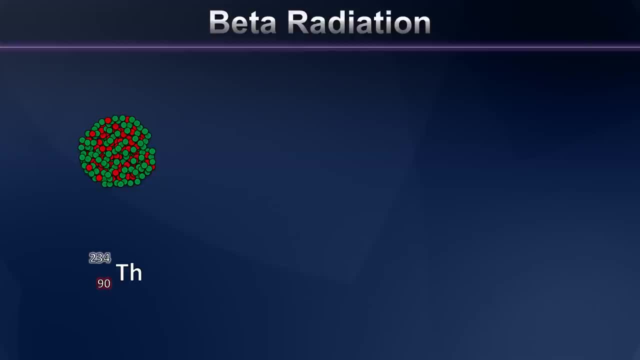 order to do that, it has to get more protons per neutron. Now, how is that possible? Well, think again about that equation that we derived earlier, in which a proton plus an electron essentially equal to neutron. Well, that means that thorium could actually convert one of its neutrons into a 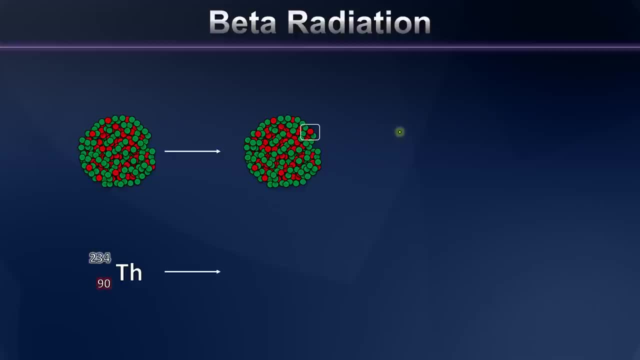 proton if it releases a high-energy electron known as a beta particle. Now look carefully at our equation here. Our beta particle has essentially no mass and a negative charge, and therefore we create a new element called protactinum. This is the second step in 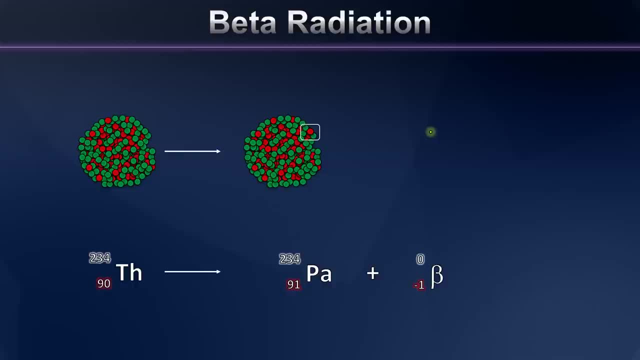 the decay of uranium, A thorium nucleus loses a beta particle in an attempt to recover the neutron to proton ratio that it once enjoyed when it was uranium 238. So in this case, we've lost a much less massive and negatively charged type of radiation as our nucleus continues to decay. 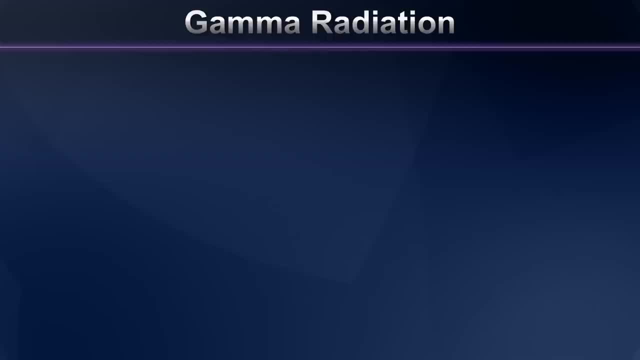 Now let's talk about gamma radiation, and to do that, I'm going to go back to our original nucleus, the uranium 238.. You see, when uranium 238 undergoes an alpha decay, it doesn't just lose an alpha particle, it loses something else. 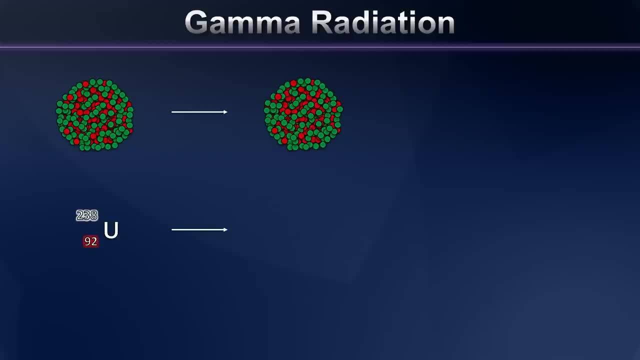 So let's think about it once more. Uranium 238 loses a helium nucleus or an alpha particle to create a massive positively charged radiation, and that creates thorium 238.. But that thorium 234 isn't totally happy yet. Just like the electrons in a 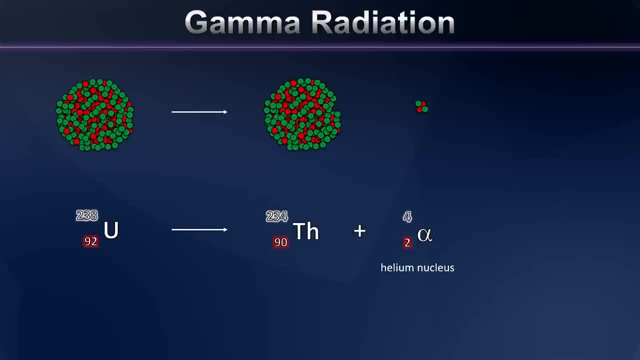 cloud around an atom like to relax to find a ground state, so do the nucleons, those protons and neutrons within that thorium atom want to relax to find their ground state, and right now they're not in it. So as they rearrange to find that, 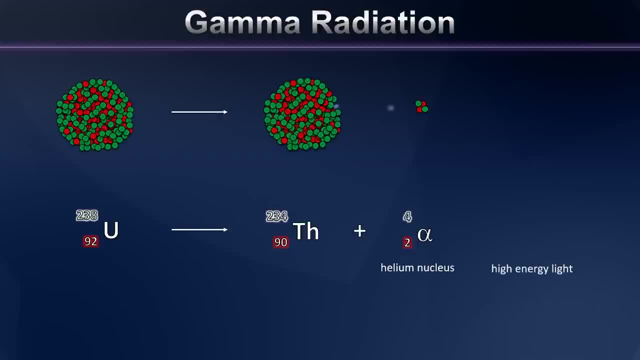 ground state, they release a certain amount of energy, and the amount of energy that they release is actually quite tremendous for a single atom. In this case, they release so much energy that a photon is released of such high energy that we call it gamma radiation. This is far, far beyond the